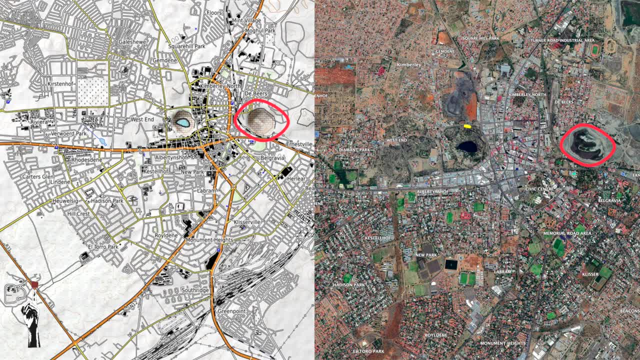 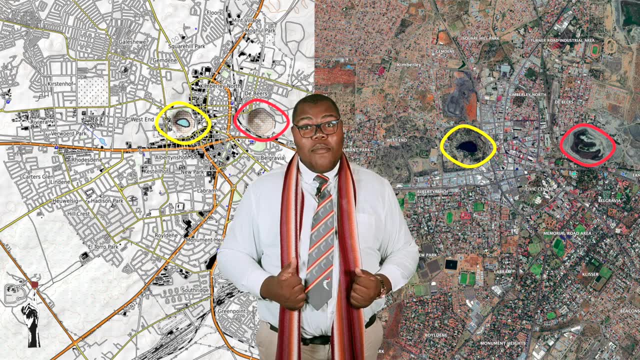 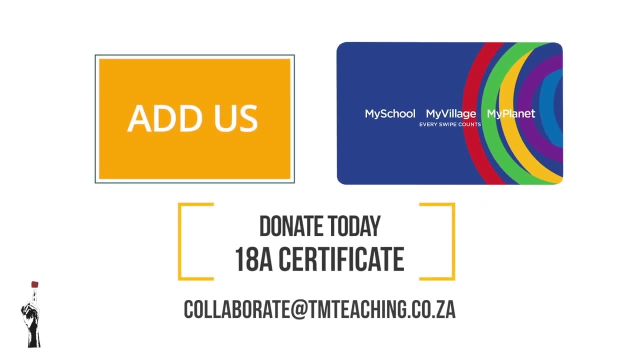 the satellite image And, as you can see, all the features we can see on the satellite image are represented on the topographical map. This allows us to be able to read the map more easily. And now, following on our little trip to Durban in lesson one, I'm now going to ask Leo. 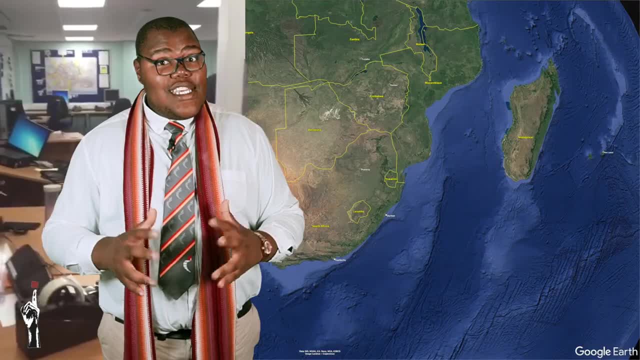 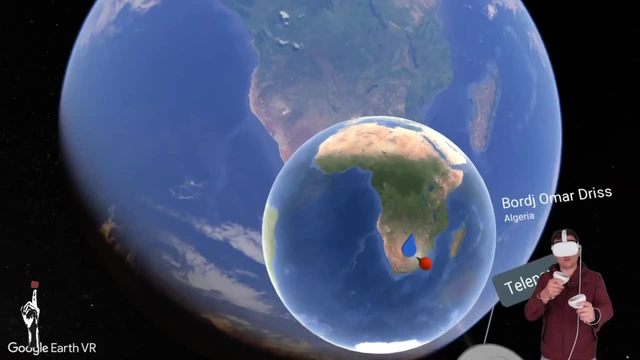 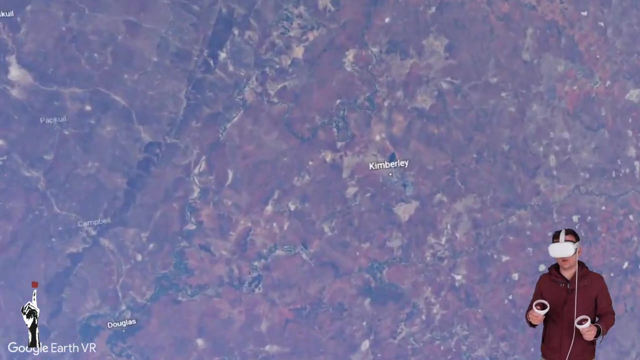 my VR pilot to take us around Kimberley to see how the features in Kimberley are represented on a map. Thank you, Mr Ntrubu. I am off To Kimberley. Let's have a look. So while I'm traveling to Kimberley. 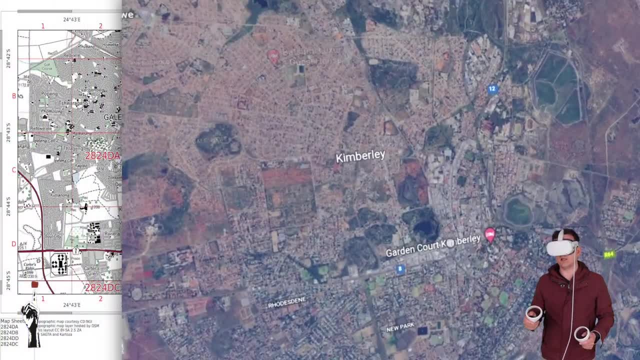 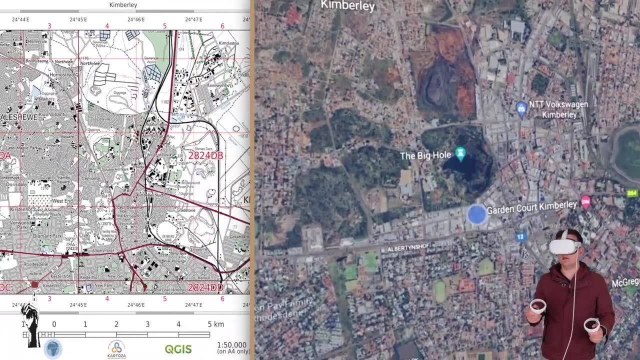 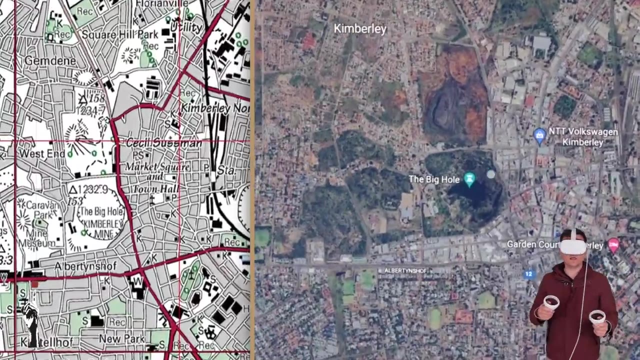 what is the whole idea of this VR pilot? The idea is for you to get acquainted with the reality compared to that what you see on the topographic map. so, as you know, you will know about the big hole in kimberly and look at it in reality compared. 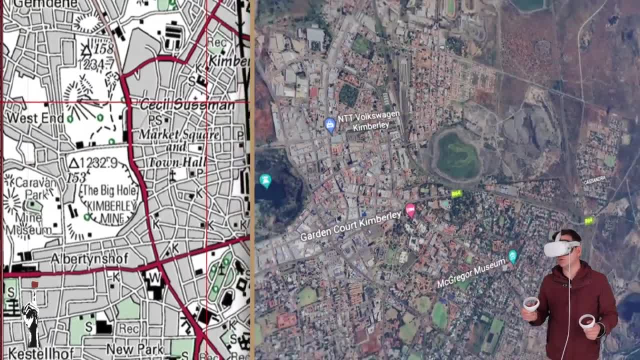 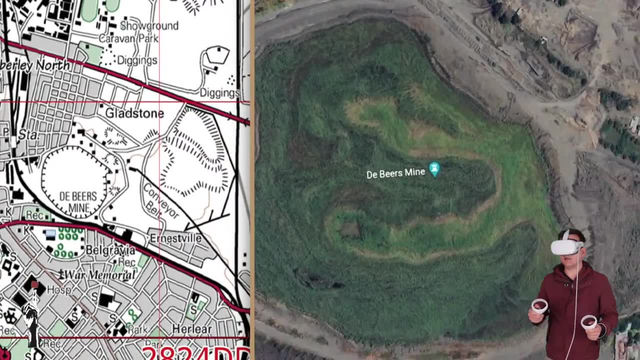 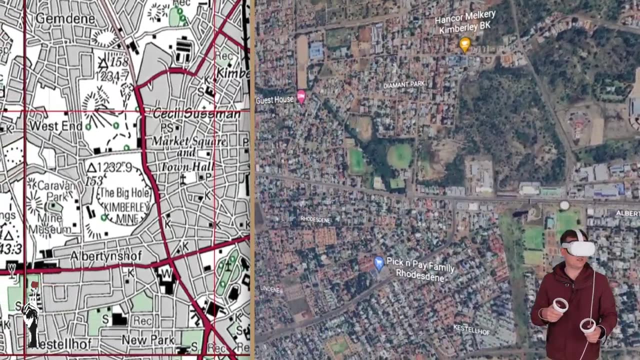 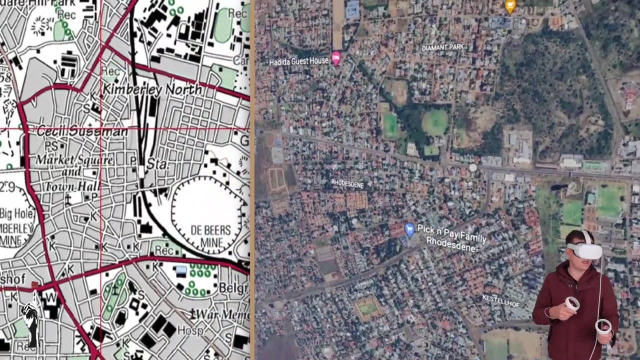 to how it looks like on the map. and also this is: i assume this is um. this is some diggings a mine. here we go and um, this looks like a national road, so this should be um. this should be read on the topographic map, and i think this is the n8, if i remember correctly. so this is the. 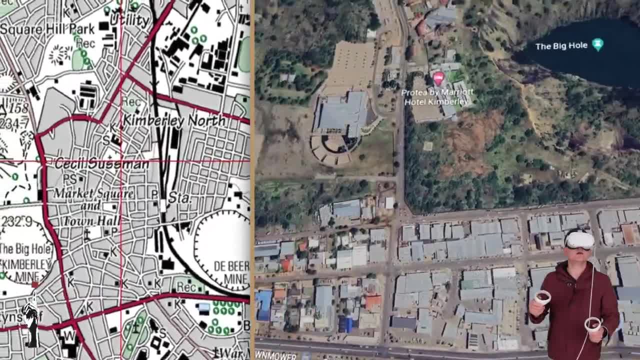 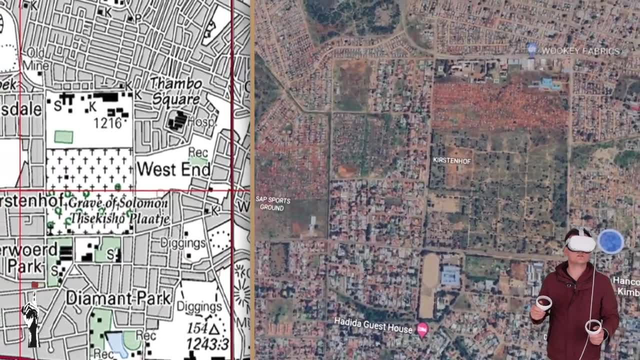 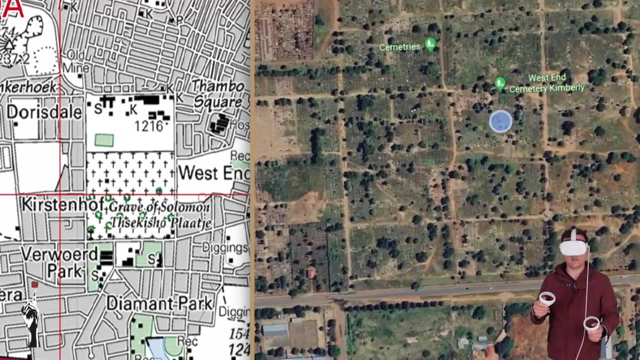 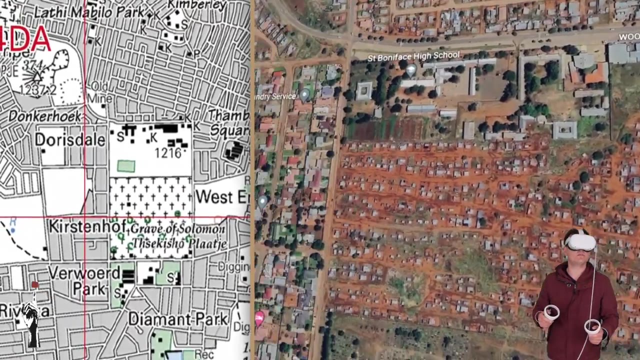 n8 or national road, and this should be red. um, let's have a look. what we, what can we see here? this looks like a graveyard right. um, yes, this is a graveyard, and i think it should display as little crosses on your topographic map right. and then one can look at the residential areas. 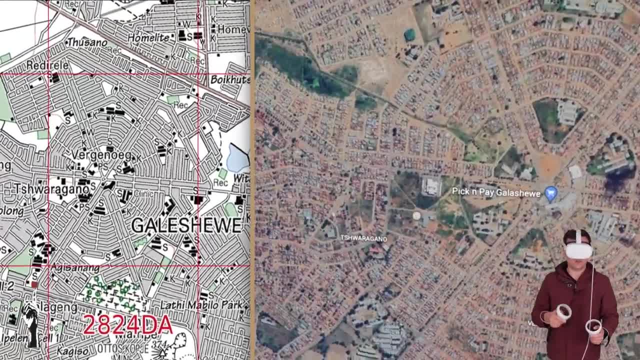 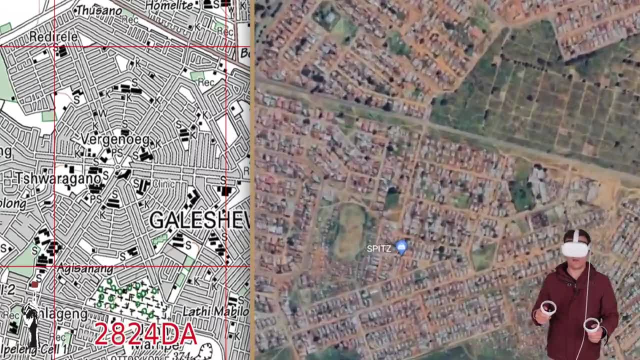 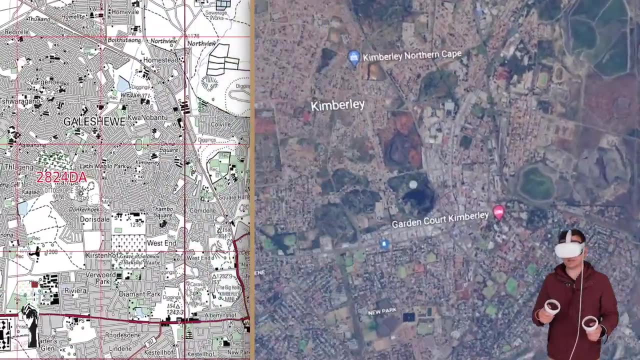 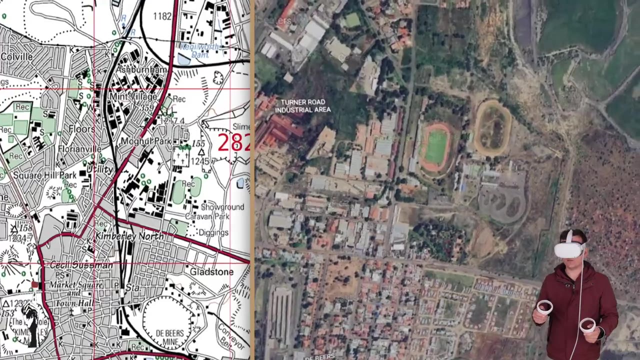 there's a unique circular or interesting circular pattern that we see here, and this is the residential area that should be gray blocks on your topographic map. so this is all just uh features that i'd like to show you and and you would like to compare this, or it will be good if you compare this with. 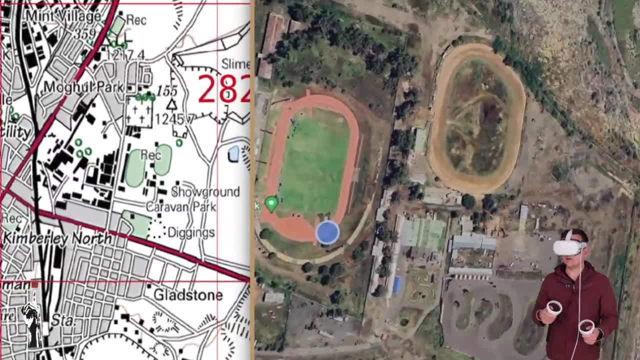 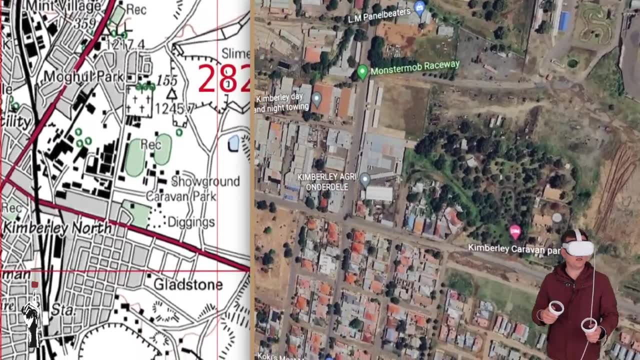 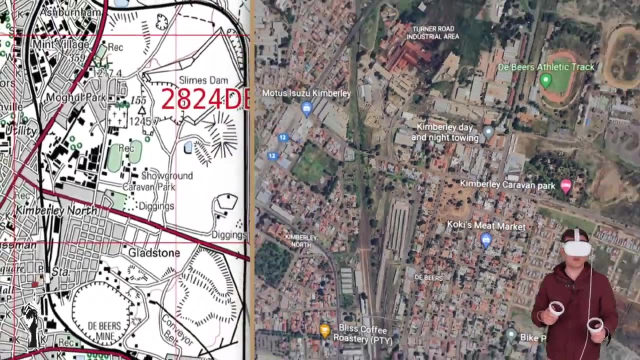 what you see on the topographic map. here's an athletic track. this looks like a racetrack. um, this looks quite interesting and, yes, that is a caravan park. and this is a quick tour of kimberly and i hope you were able to identify the realities. 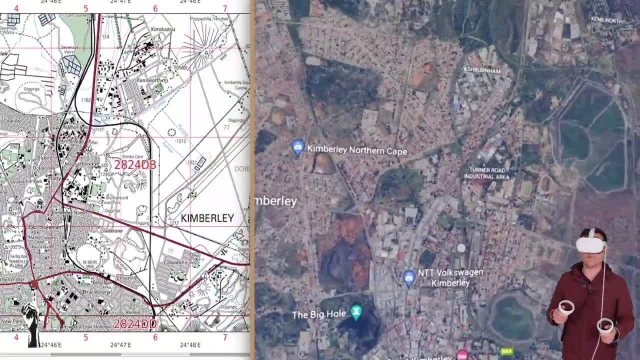 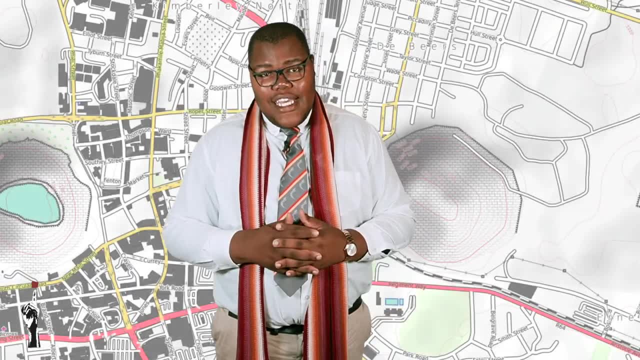 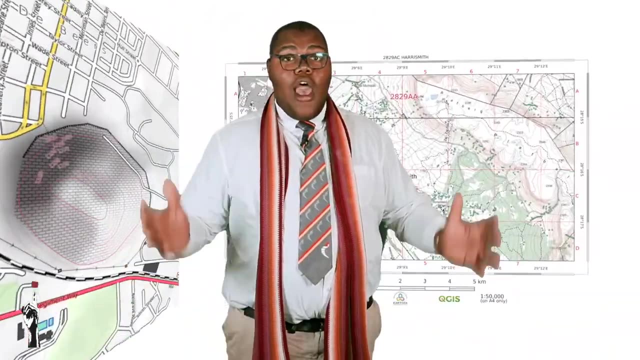 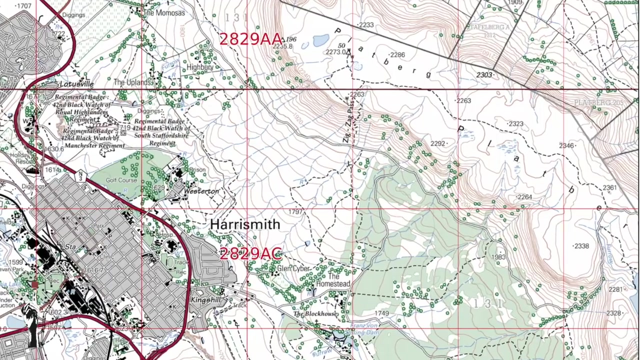 compared to that which you see on the topographic map. all right back to you, mr mtubu. thanks, leo, that was great. i hope you are able to see how the topographical map represents the geographic features on the ground. topographic maps are essential tools. they're essential for explorers, hikers and geologists, land management and for planning. 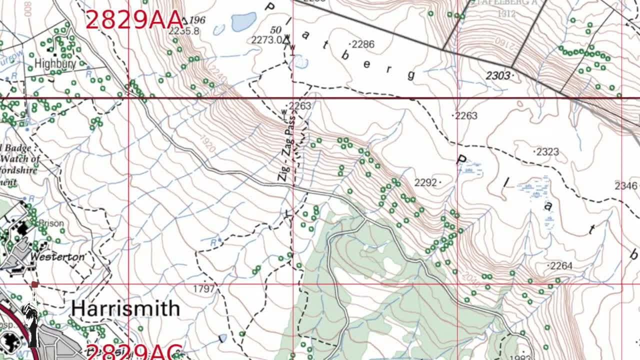 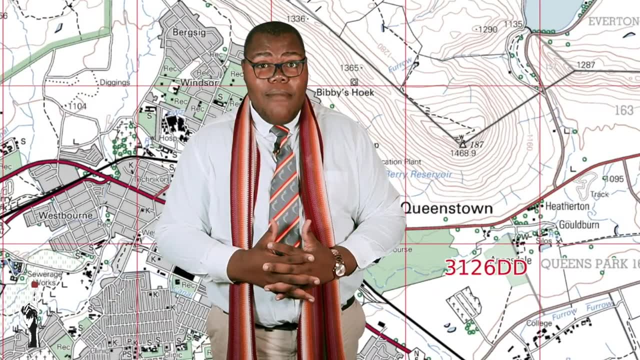 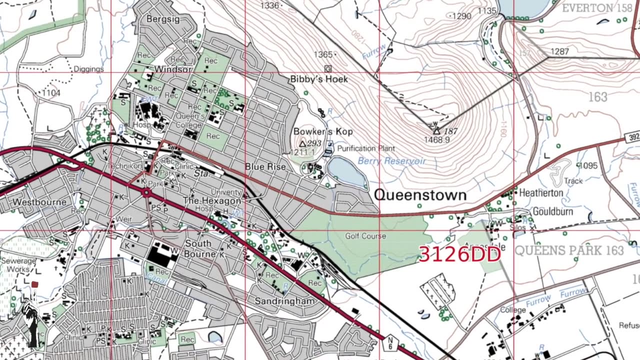 people who need to navigate and understand the terrain of an area. in this video, we will learn about the key features of a topographical map and how to read a topographical map. so let's have a closer look at topographic maps. these maps show the physical and artificial. 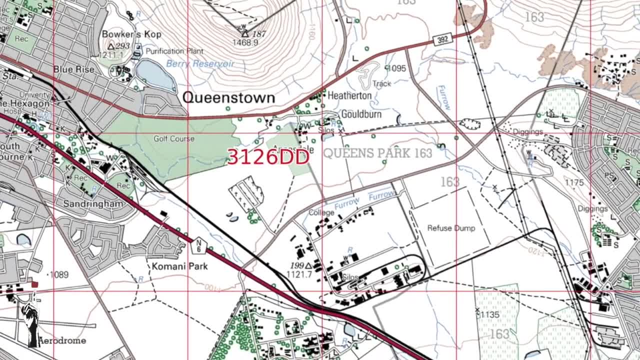 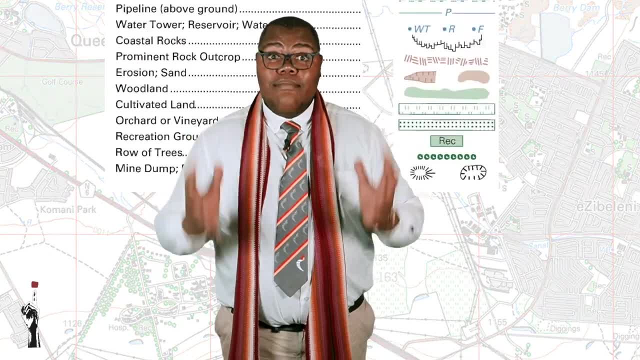 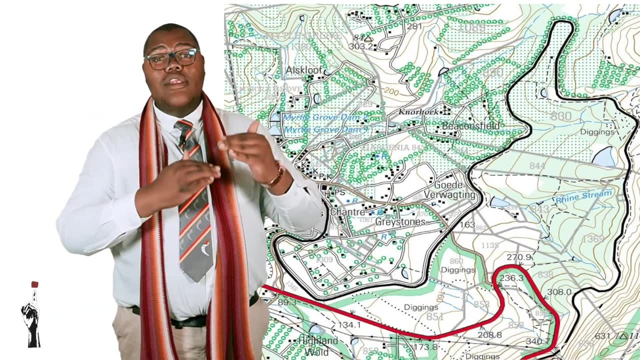 spatial features of an area, such as buildings, monuments, mountains, valleys, rivers and other natural and artificial forms, and it uses symbols as well as color to convey information. take a look at the following map, where we are going to break down all the information by color for you. okay, now we're going to separate the colors. 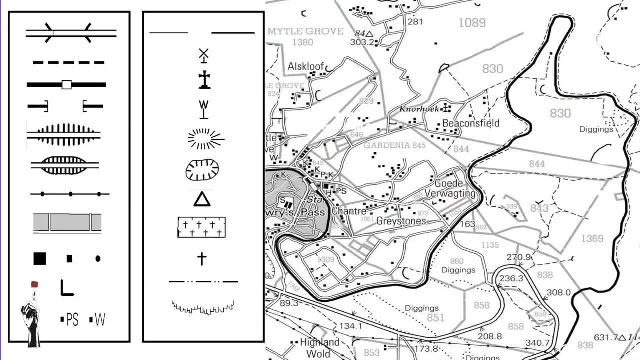 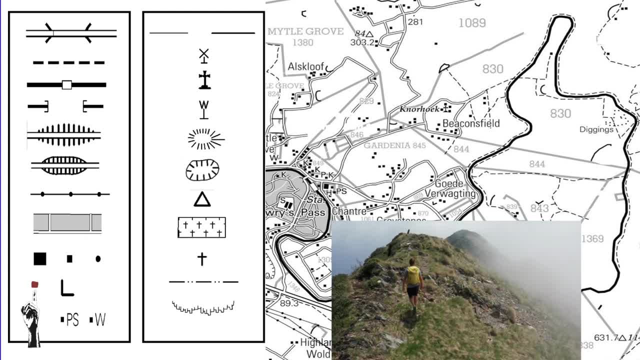 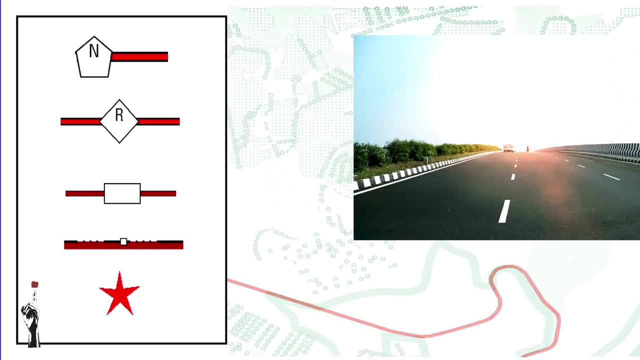 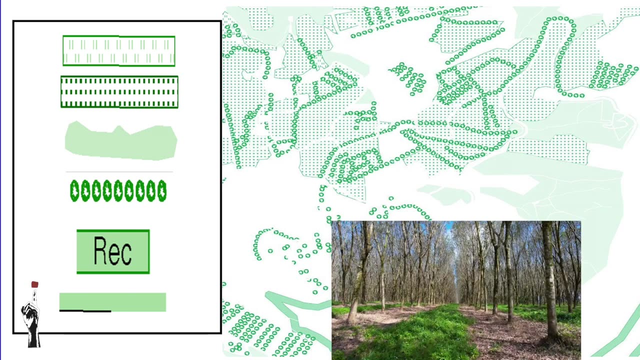 we have black representing everything that is artificial. so you'll see that the power lines, the hiking trails, the walls, they are represented by black. then there's red. red represents the national roads. green represents everything that is planted. so this is green. green represents our vegetation, trees, cultivated lands will all be represented. 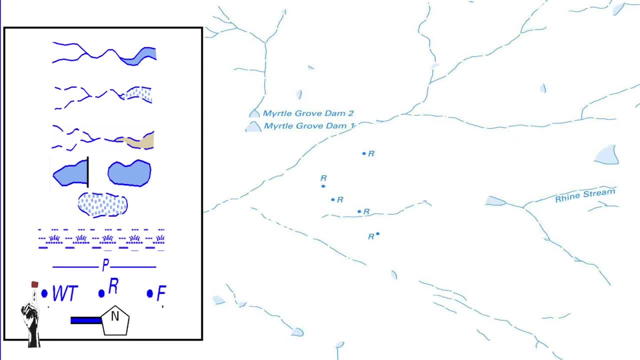 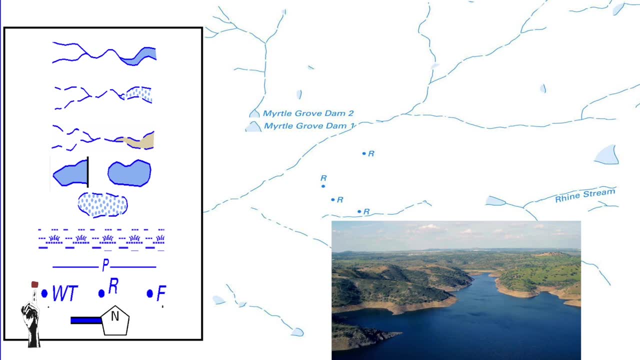 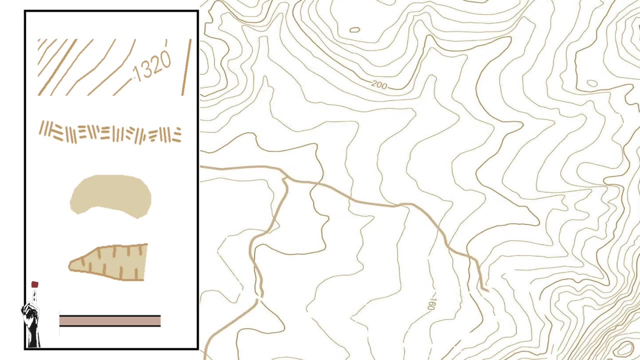 by green, then blue everything that has to do with water. so all water bodies, rivers, dams, lakes, will all be represented by blue and finally brown brown. we'll see the lines on the map. a brown brown represents contour lines right, and contour lines help us to quantify elevations and represent group and we're going to talk a little bit about these orange dots now. we're going to see some of them. we're going to see this one is percentage and we can think about the heat used to measure. and finally, flavors and colors of the water. we're going to just go through as we go along. 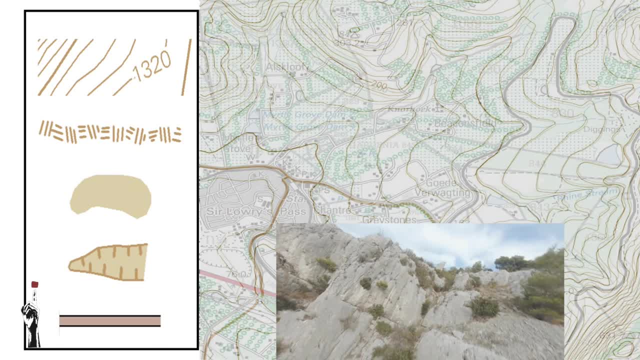 alright. so it's true that here we have aitu聊くinos, the trees, and we explore the class of plants. then we bring the value of grass and we bring the size of plant comparable soil and we eliminate the elevation And put together- voila, you have loads of information. 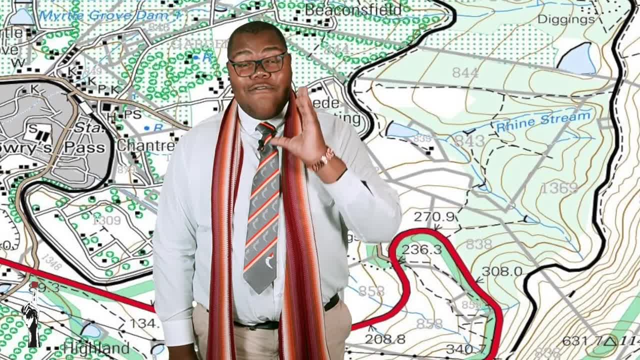 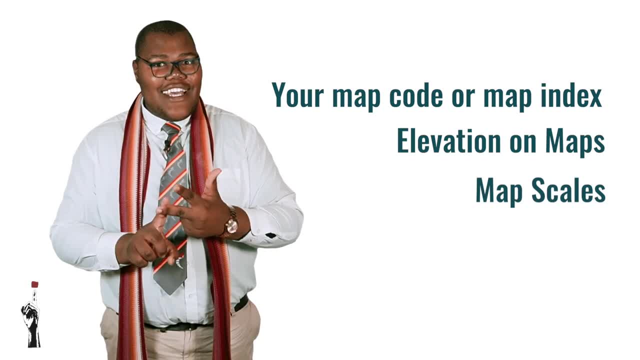 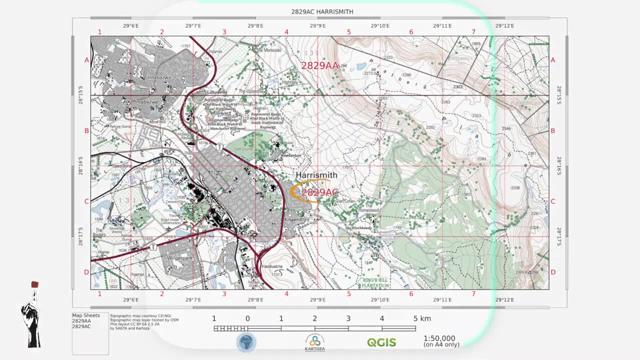 Now I'm going to run through some important aspects of topographic maps. We're going to run through map codes or map index, elevation on maps and map scales, Starting with your map code or map index. All maps have a map code or map index. Think of the index of a. 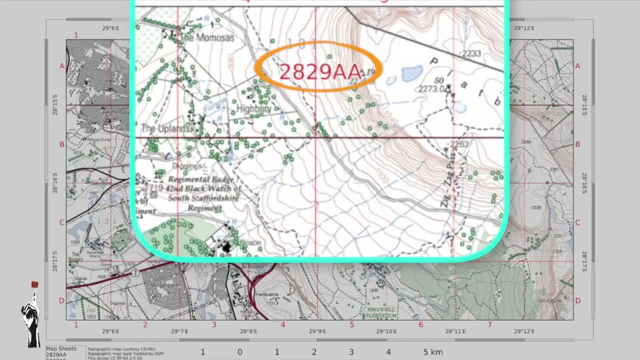 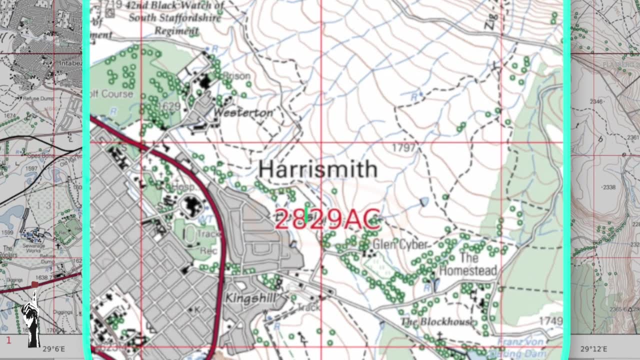 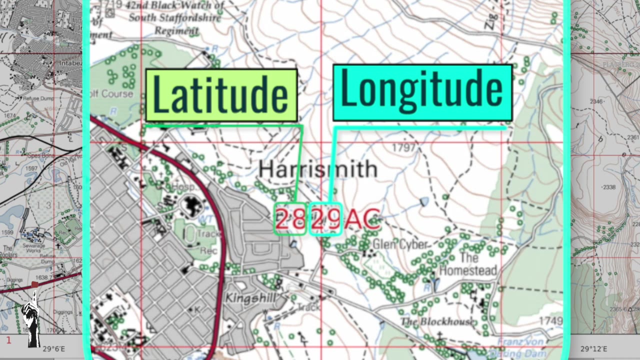 book. That's exactly what this index is. It is the specific location of the mapped area in relation to others. The first two numbers refer to the latitude of the mapped area and the following two refer to the longitude. There's a special way to figure out how the 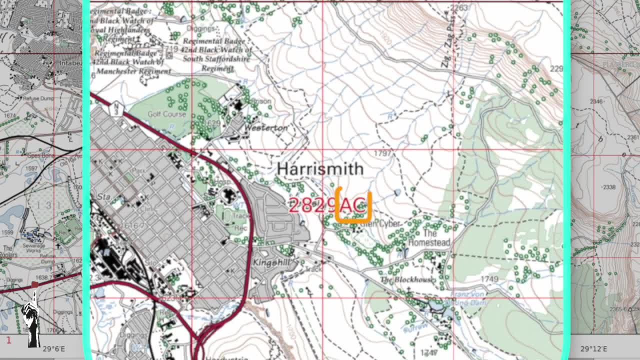 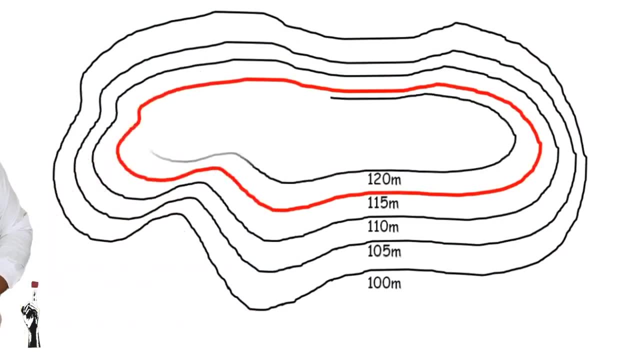 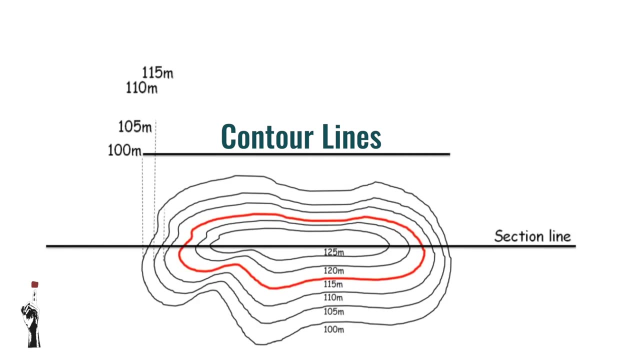 two letters are calculated, but that's a lesson for another day. Now, moving over to contour lines, which are the imaginary lines that join places of equal height. Contour lines are curved lines that connect points of equal elevation on a map. They help us visualize the shape and steepness of the terrain. The closer the contour. 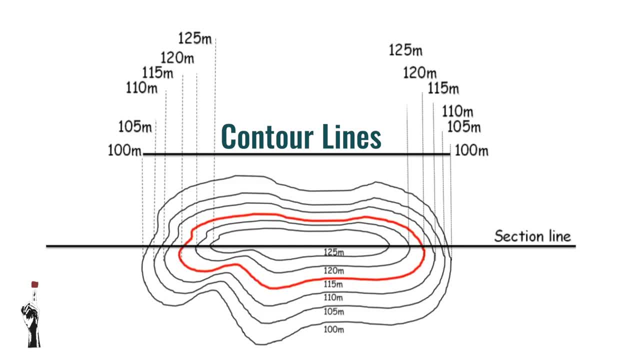 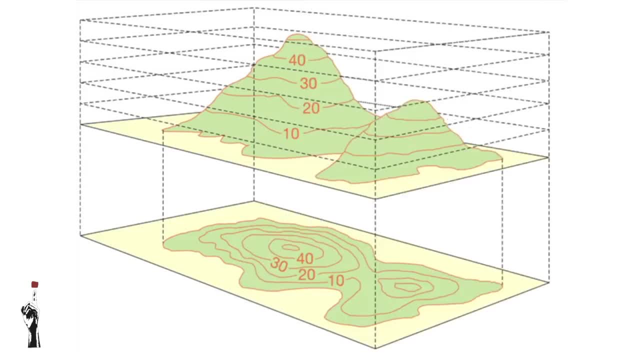 lines, the steeper the terrain. The further apart the contour lines, the flatter or more gentle the terrain. And this is important because we are able to perceive the elevation and shape of the terrain even by looking on a flat piece of paper. 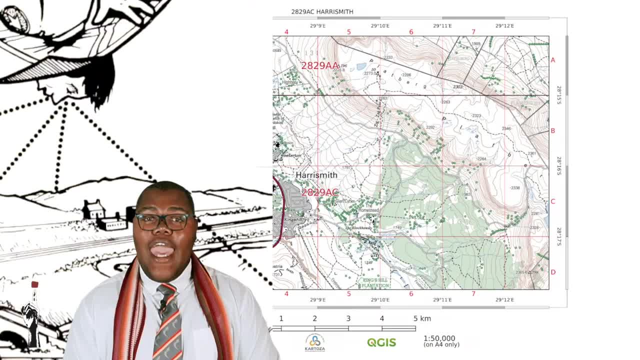 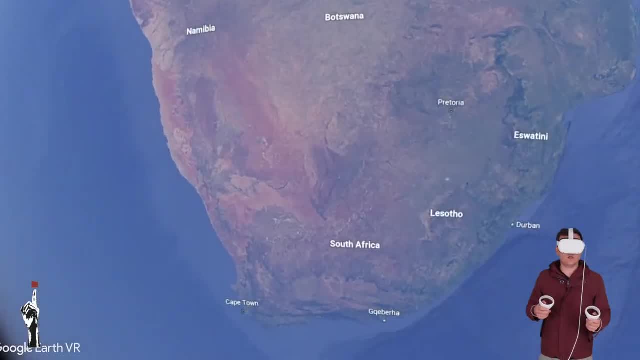 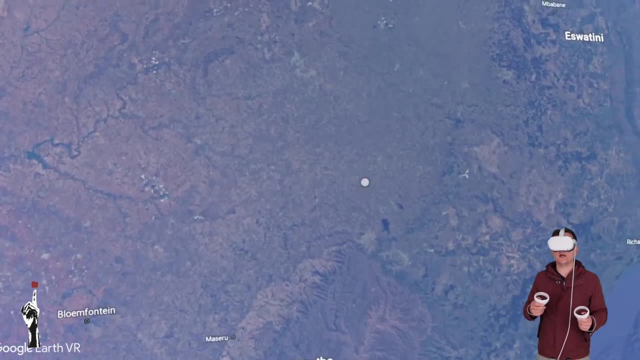 Alright, I think this is a good time to get to our pilot. Hey, VR-pilot, could you please take us to an area that is steep and also flat? OK, so, as we are discussing contour lines, I would like to take you to Harry Smith, which. 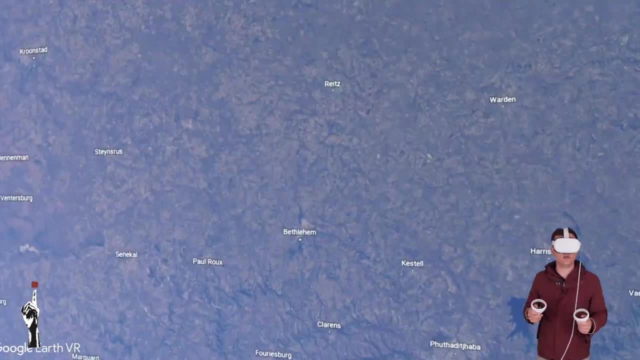 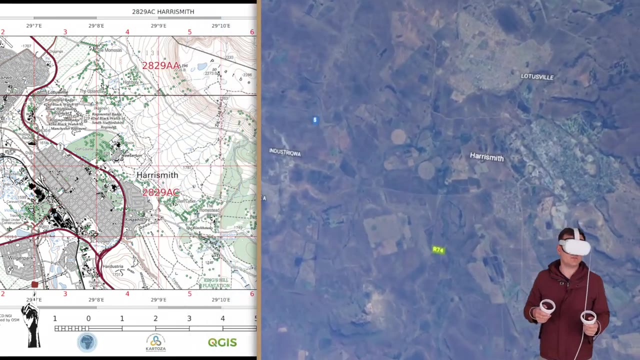 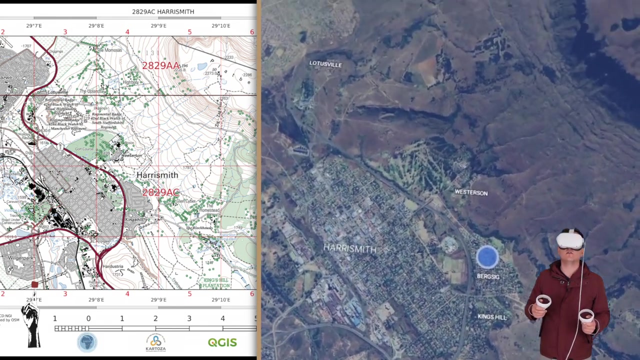 is just North of Lesotho, In this area, somewhere here. There we go. there we go And have a topographic map of Harry Smith next to you And the idea is to consider this area and the contour lines that you can see on your topographic map. 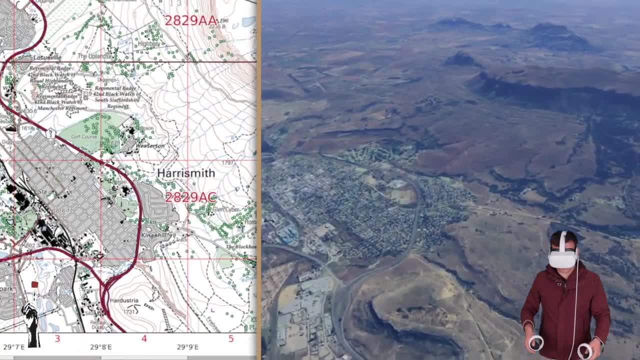 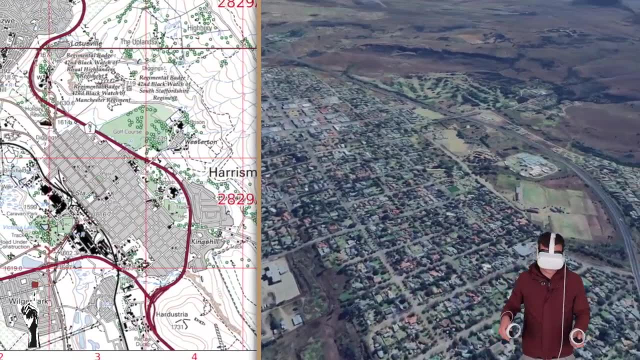 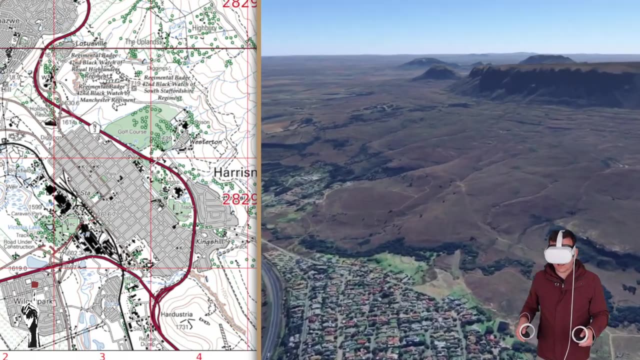 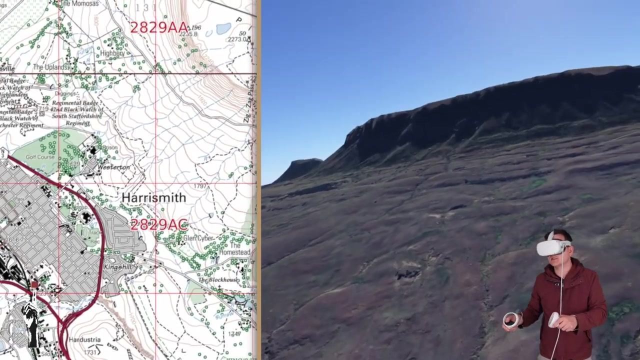 So let me fly into this area in here. Okay, now note that the town area is pretty flat, as you can see, And so the contour lines should be quite far apart from each other. But then, as we fly to the mountain, we can see that it gradually gets steeper as we get closer to the mountain. 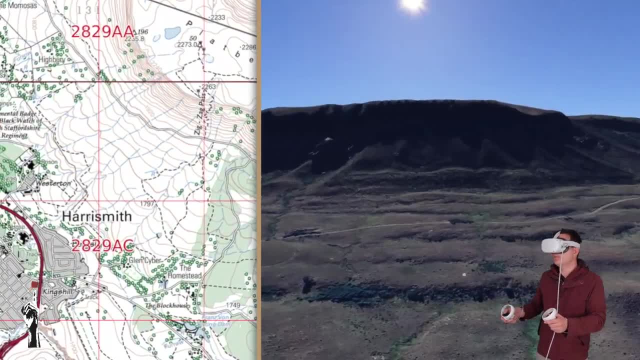 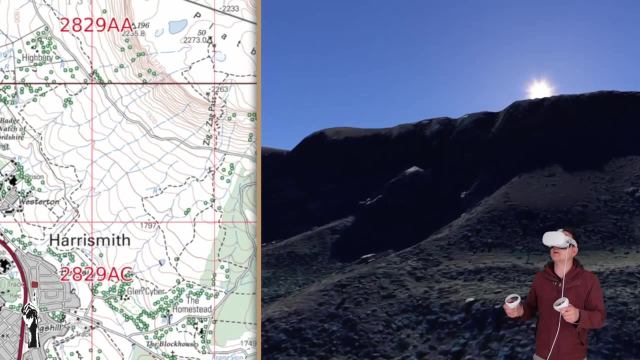 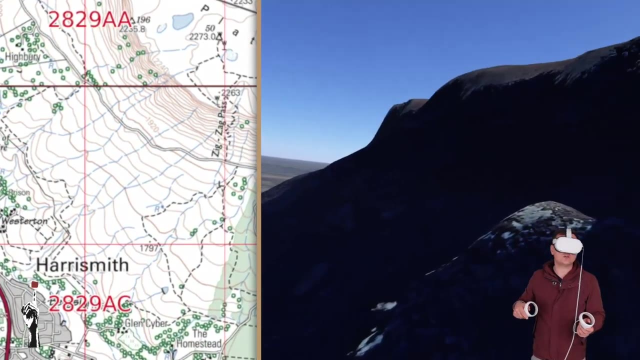 So there should be some contour lines that are gradually coming closer to each other, And now it should be very close to each other, And as we reach the top of this mountain, there should be The contour lines, should be all getting closer together. 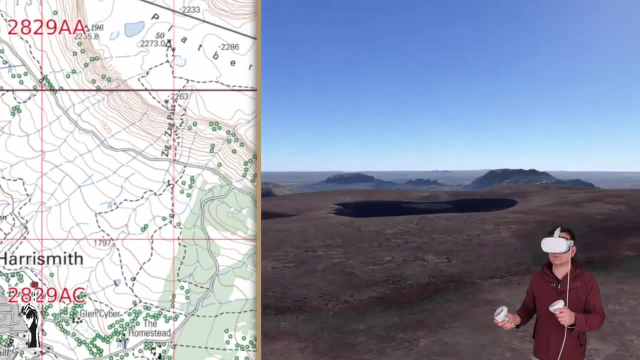 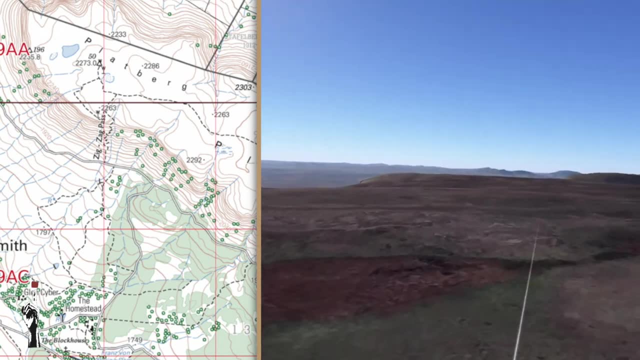 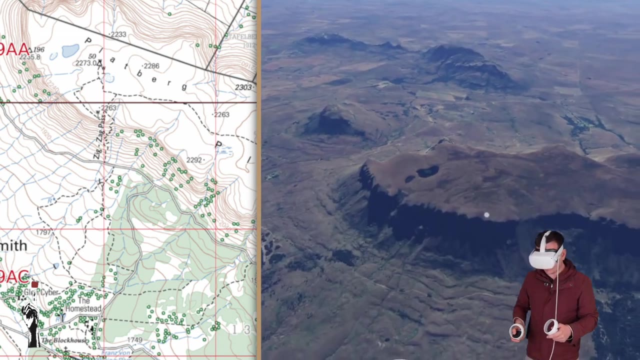 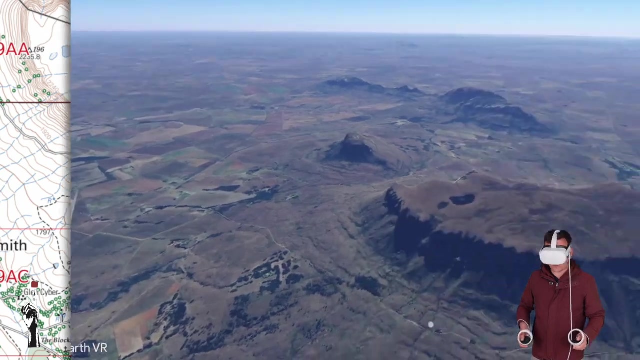 And as we reach the top, it's very flat, this plateau area right. So, yes, this is just a quick demonstration of an area that we can investigate, the contour lines of a topographic map. Thank you. Back to you, Mr Mtubu. 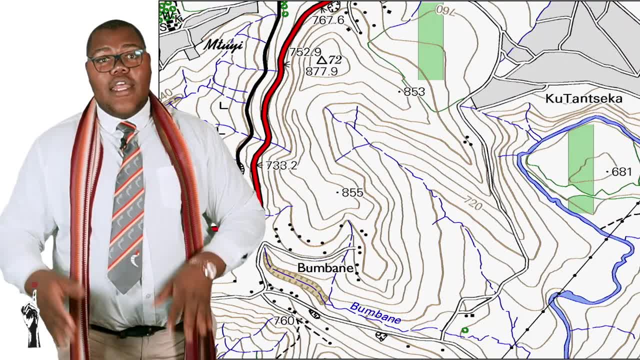 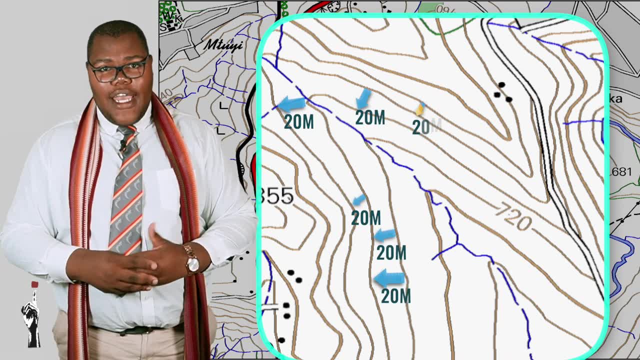 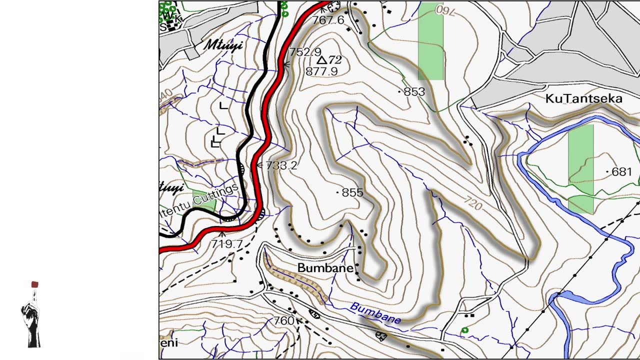 Now for the maps that you guys will be working with. they have a contour interval of 20 meters. Contour interval means the difference between each contour line is 20 meters. Every 100 meters will be a bold contour line. Now, contour lines is one of four ways to indicate height on a map. 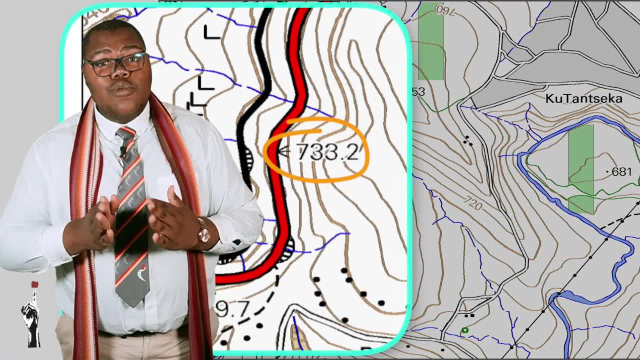 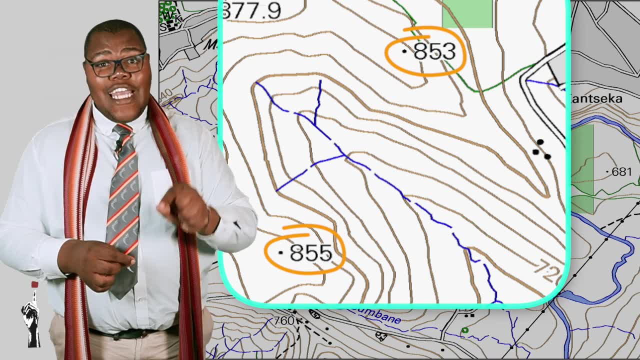 We can also have a benchmark, which we'll normally find along the road, Or a spot height, which will be on any random spot on the map, indicated by a dot and a number next to it indicating the height at that particular position. 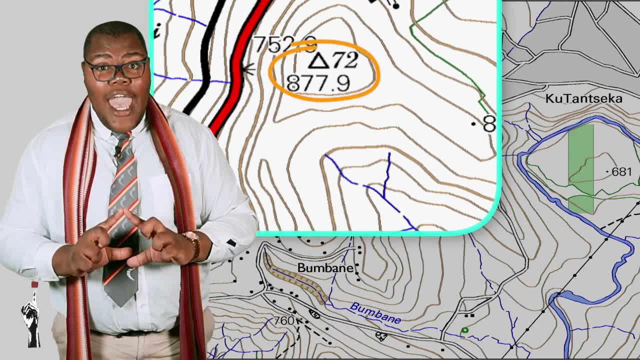 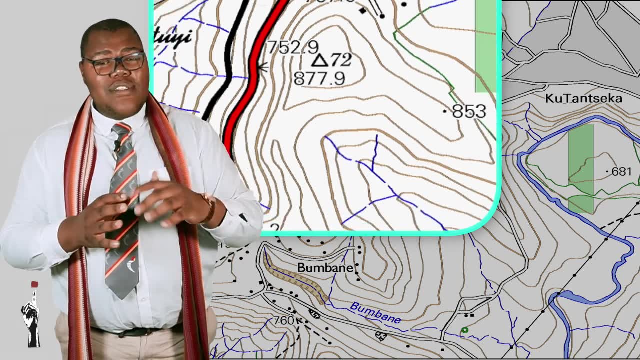 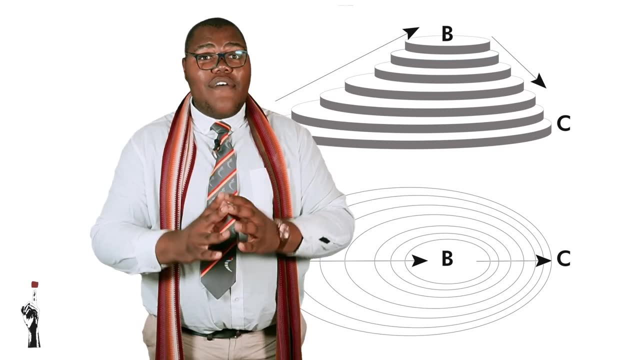 We can also have a trig beacon, which will look like a triangle on your map, with a beacon number and the height just below it, which is normally found at the top of mountains or hills, As I mentioned earlier on, contour lines don't only give us height, they also give us shape of geographic features. 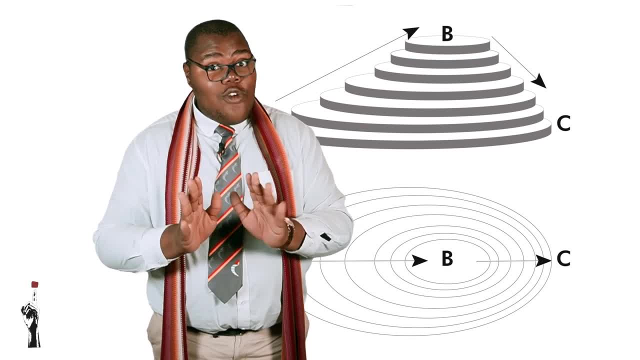 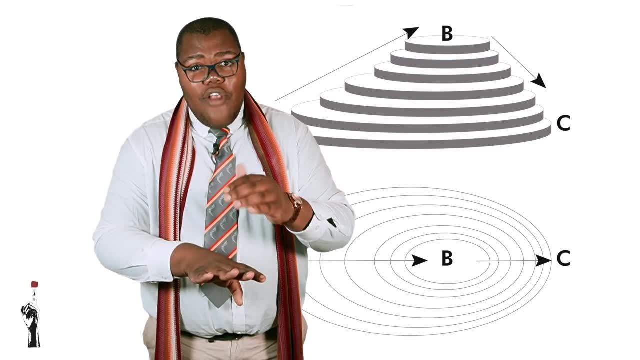 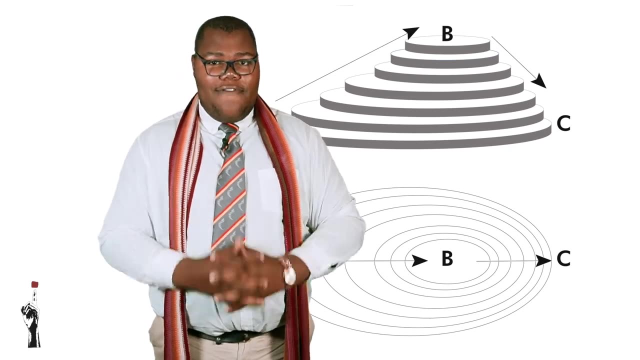 Now, in order to see this in reality, what I normally do with some of my learners is to take little glass offcuts, little glass tiles, and trace every contour line on the map. Stack the different cuts together. They will give you the shape of a feature. 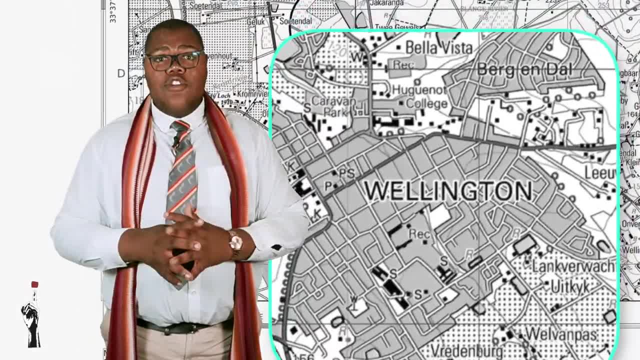 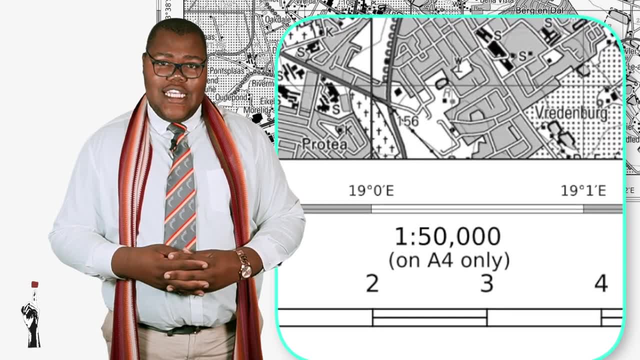 Moving over to scale. Most of the maps that you'll be dealing with will be topographical maps with a scale of 1 is to 50,000.. What this means is One unit on the map is 50,000 units larger on the real ground. 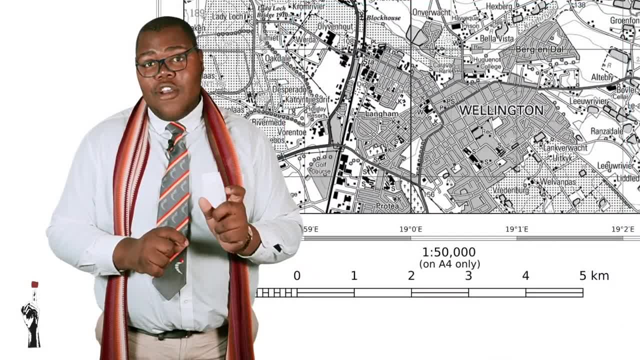 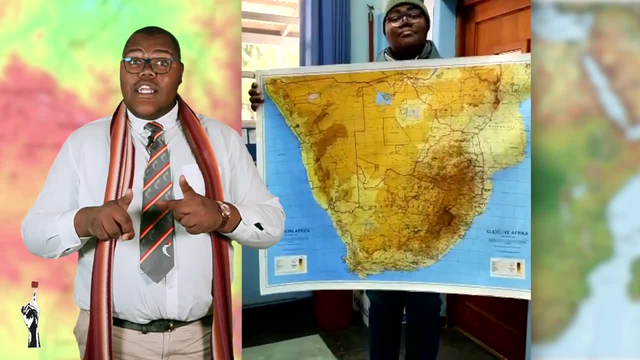 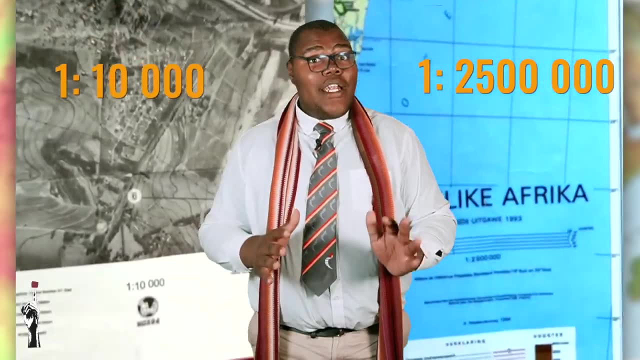 So this technically means that every one centimetre measured on your map is equal to 50,000 centimetres on real ground. Here's an example of a map of 1 to 2.5 million. Here's another example of a map of 1 to 10,000.. 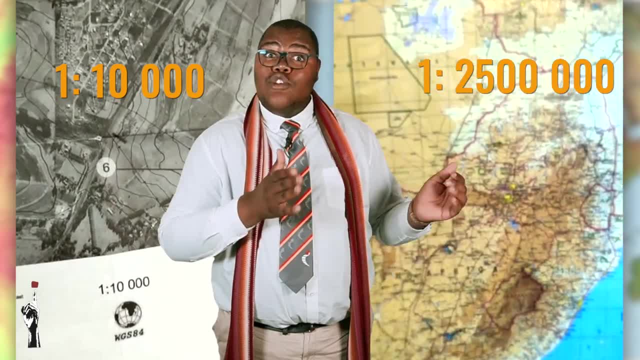 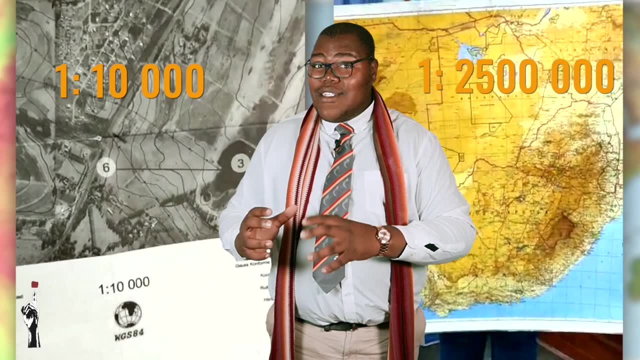 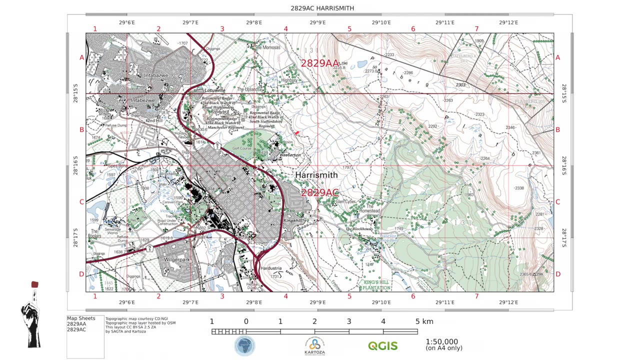 Can you notice anything on these maps? The 1 to 2 million covers A larger area, but into very little detail. Yet the 1 to 10,000 covers a smaller area but in greater detail. There are different types of scales, including line scales, where a straight line on the map represents a certain distance on the ground. 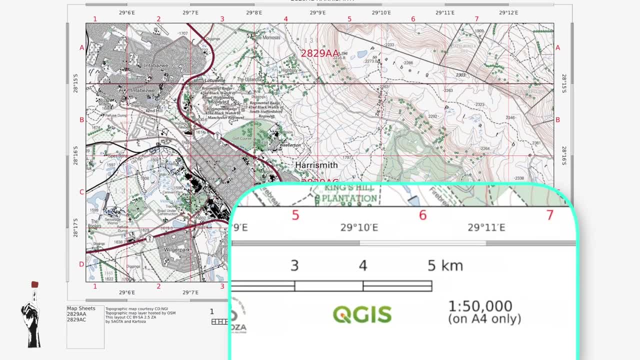 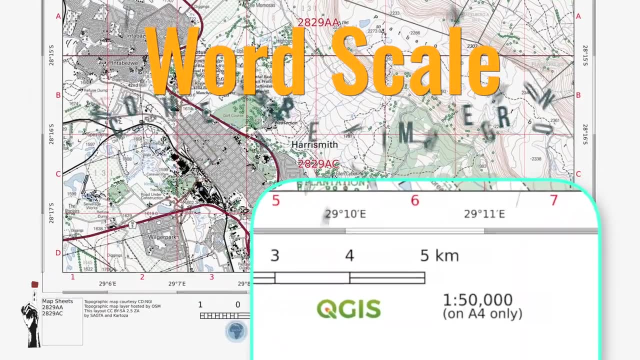 There are also ratio scales, where the scale is expressed as a ratio, such as 1 is to 50,000.. And we also have word scales, where distances are given in words. For example, the length of the map is 1 centimetre and the length of the map is 1 kilometre. 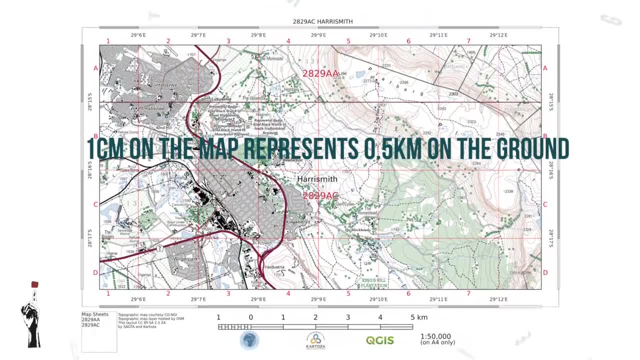 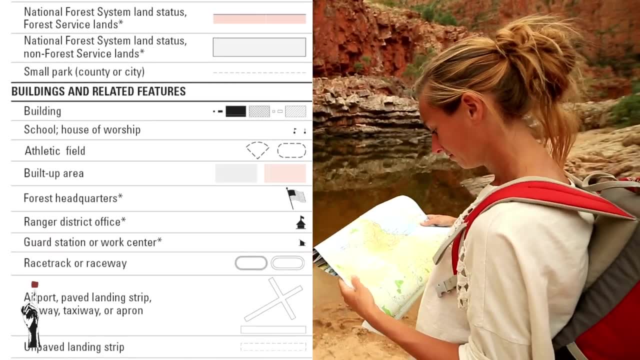 Or, in the instance of a topographical map, 1 centimetre would equal to half a kilometre. It is important to know how to read a topographical map, to understand the terrain and to plan your route. Let's take a look at an example. 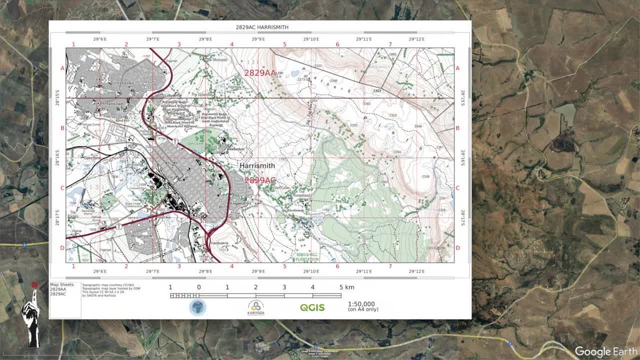 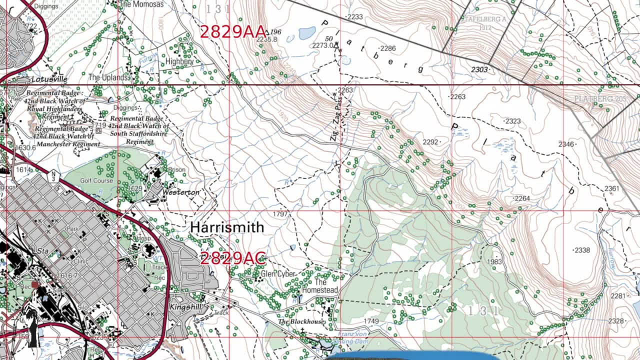 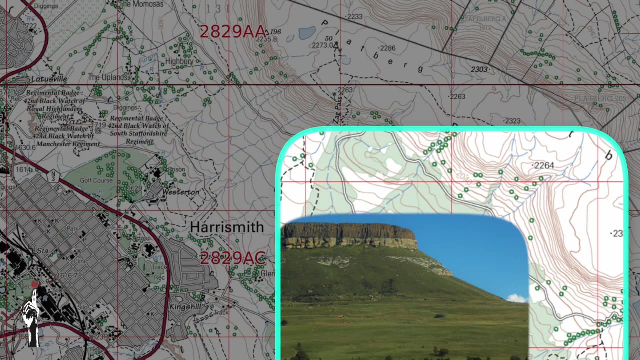 This is a topographical map of the Platberg mountain, which is in the Eastern Free State in South Africa. The contour lines on this map show the elevation. as I mentioned earlier on, The closer the lines, the steeper the terrain. The Platberg mountain is a popular hiking destination and the map is useful for planning a hiking route. 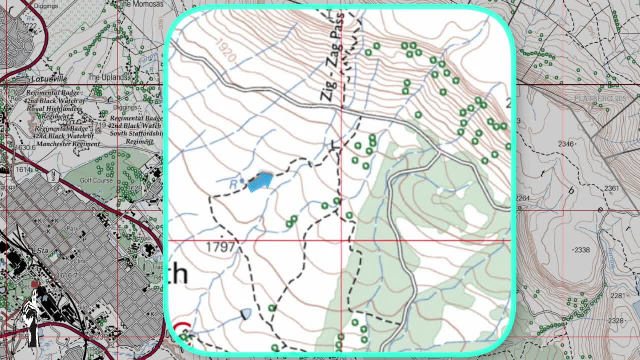 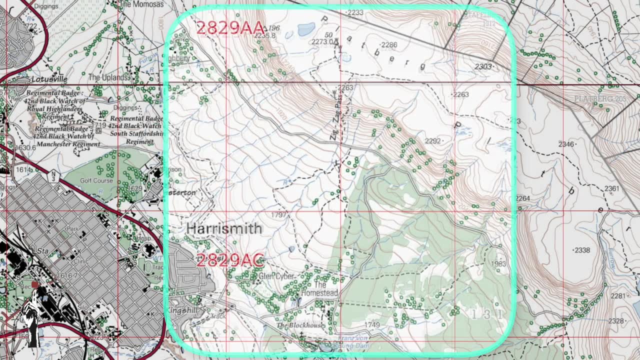 The black dotted lines on the map indicate hiking trails and the green areas show vegetation. The blue lines on this map show rivers and water bodies. So when planning your route, you need to look for the contour lines. So when planning your route, you need to look for the contour lines.